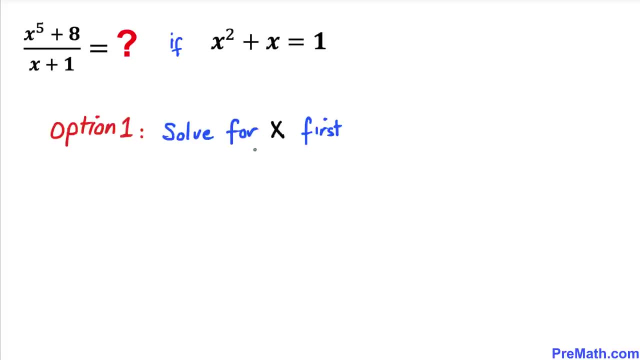 let's go ahead and talk about couple of options. And here's our very first option: solve for x first and then find the value of this rational expression. And here's our second option: look for an easier alternative approach to avoid solving for x first. So I have decided to take this. 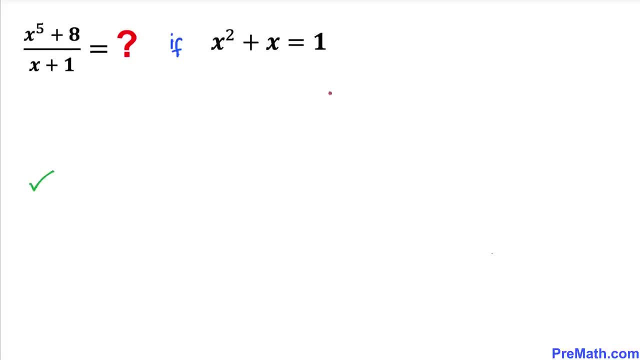 second option and we're going to think outside the box. And here's our very first step. Let's focus on this equation. I'm going to call this equation as number one. Now let's focus on this equation, And here I have copied: 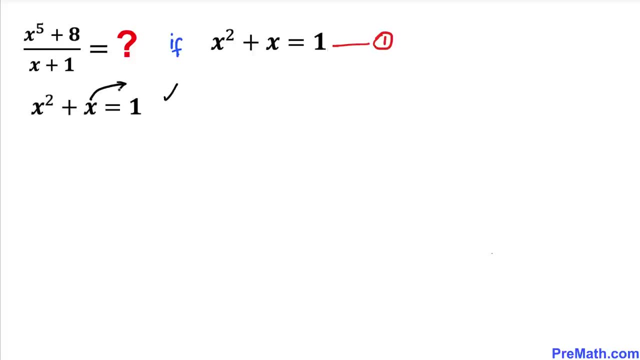 it down. Let's go ahead and move this x on the right hand side, So this equation is simply: is going to become x square equal to 1 minus x. Go ahead and call this equation as number two. And now let's go ahead and take the square on both sides of this equation two. So let's go ahead. 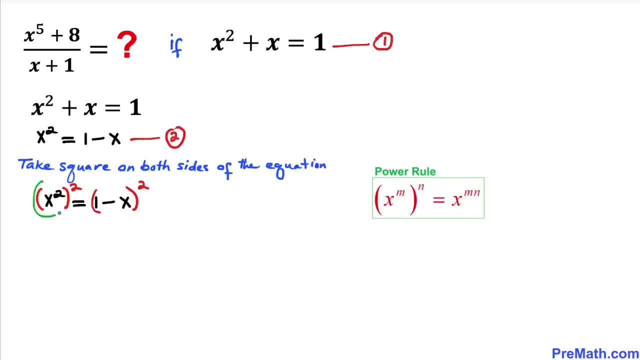 and take the square on both sides of this equation two. And now let's focus on this left hand side of this equation: x power two and then power two. We are going to use this power rule of exponents, So this could be written as: x power two times two is x, power four equals two. And on the right hand, 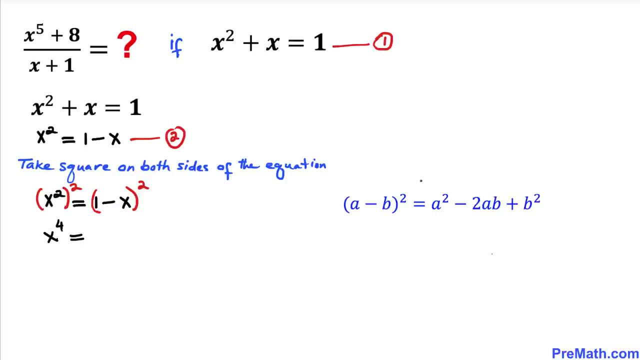 side. we are going to expand this binomial by using this famous identity a minus b square. So the right hand side could be written as one minus b square. So this is going to become a minus b minus 2x plus x square. and now let's focus on this x square term. I am going to replace this one. 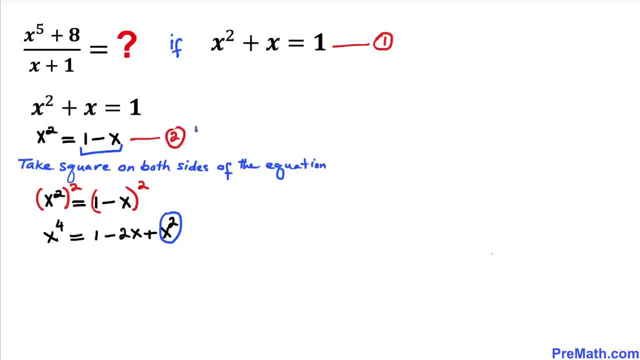 by this 1 minus x in equation 2. so therefore our this equation is going to become x power 4 equal to 1 minus 2x, and then plus. I'm going to replace this one by 1 minus x, so let's go ahead. 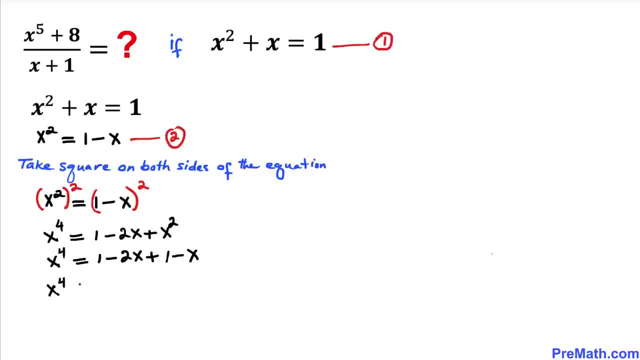 and simplify furthermore. so x power 4 equal to. let's combine the like terms on the right hand side, so that's going to give us 2 minus 3x. let me go ahead and call this as equation number 3, and here's our next step. let's go ahead and multiply x on both side of this equation, so 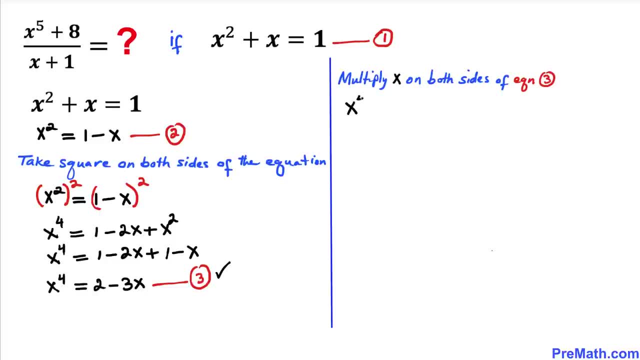 let's go ahead and do that one. so we're going to have x power 4, and then times x equals to x times 2 minus 3x. now on the left hand side, that is going to give us x power 5 equal to. let's go ahead and distribute. 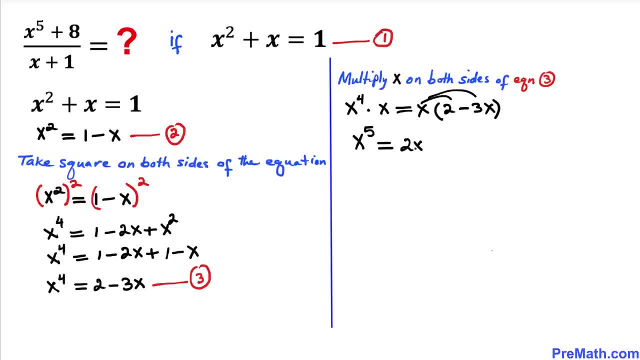 these. so we are going to get 2x minus 3x square. and now we can see on the right hand side this x square. I am going to replace this by 1 minus x as an equation 2. so therefore our equation is going to become: x power 5 equals to 2x minus 3 times. I'm going to replace it by 1 minus. 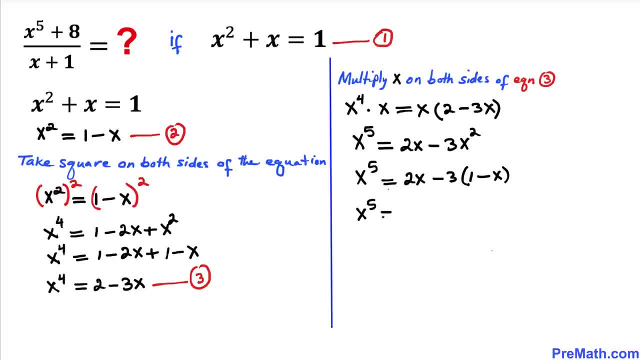 so we are going to have x power 5 equals to 2x minus. let's go ahead and distribute this thing. that's going to give us negative 3 plus 3x. so this is going to give us x power 5. let's combine. 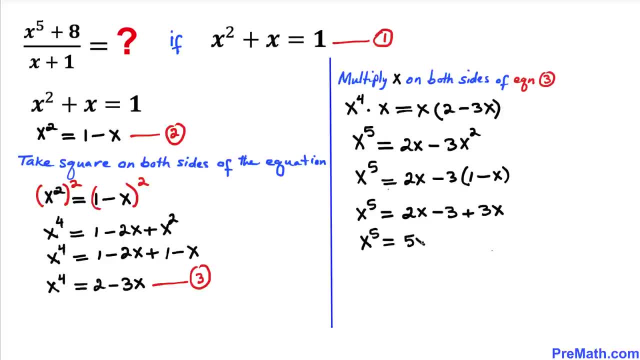 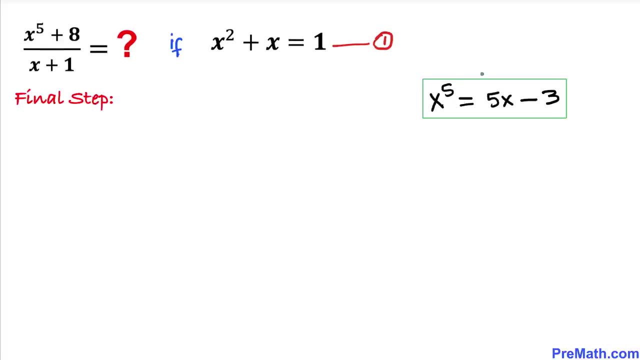 the like terms on the right hand side. that's going to give us 5x minus 3, and this is going to be our crucial component in figuring out the value of this rational expression. and here's our final step. we already figured out our x power- 5 equals to 5x minus 3- in our previous steps, and now let's focus. 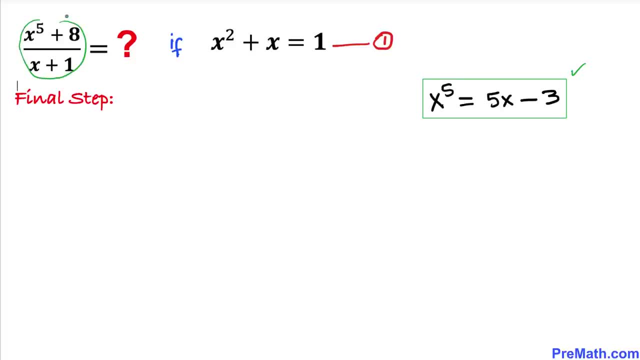 on this rational expression, and here i have copied it down and let's focus on this x power 5. i am going to replace this x power 5 by this 5x minus 3, so our this fraction is simply is going to become 5x minus 3, and then plus i'm.